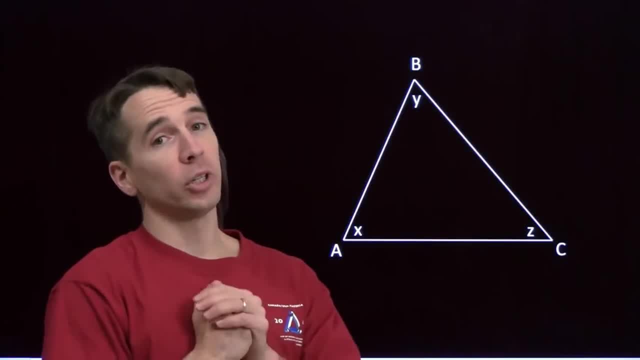 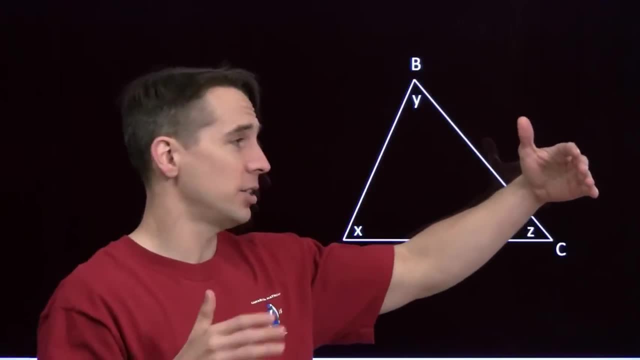 figure out how to do it, So I had to call in some very special help. I called in really good friend of mine. Come on in here, Harvey. Yeah, this is Harvey. This is my man, Harvey, My man is wicked good at geometry. He knows all kinds of geometry. He's got a very special. 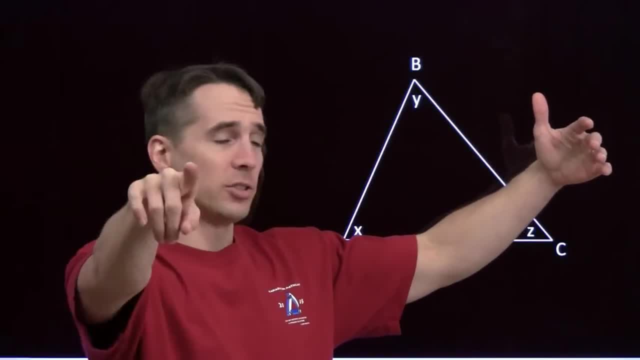 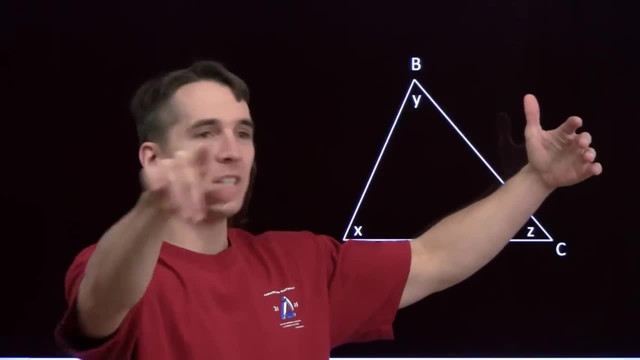 skill. So, Harvey, I want you to say hi to the students here before we get started. Harvey, they're over there. Harvey, they're over there. I know you can't see them, but they're there, I know you can. They can see us. Yes, they can see us. Just say hi, I can't take him. 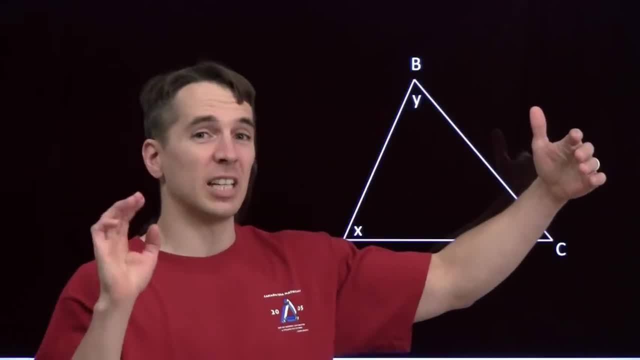 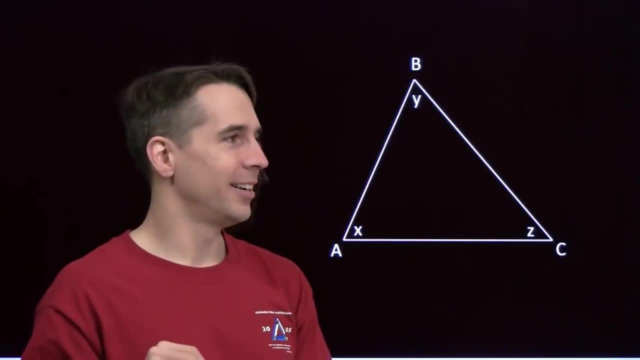 anywhere. All right, now my man, Harvey, here. he has a very special skill that's extremely useful—check this out, Harvey—in geometry problems, And that skill is seeing things that aren't there. Yes, Harvey, like the students. Okay, so here we go, Harvey, We're. 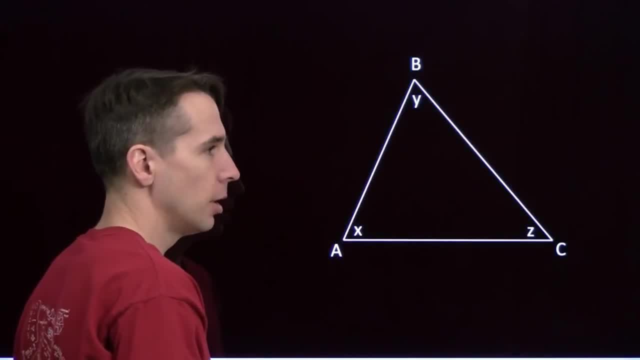 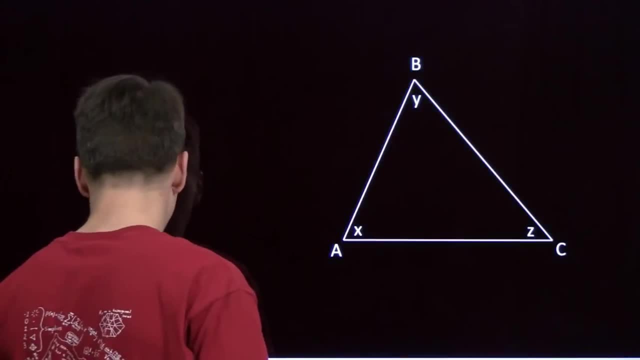 trying to prove—yeah, we're trying to prove- that the angles add up to 180 degrees. What Use the? what Use the parallel line? There's no parallel lines here. Oh, in the other slide, In the other slide. Okay, No parallel lines here either. Oh, you see one, but you want. 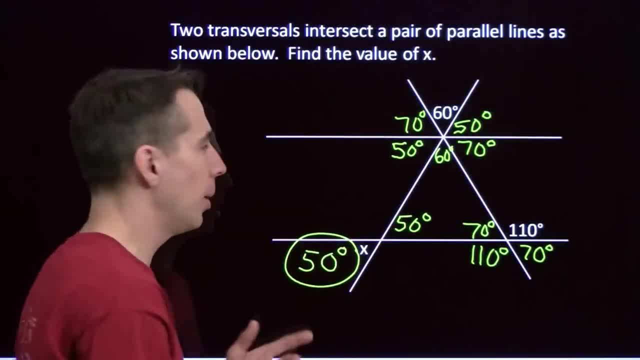 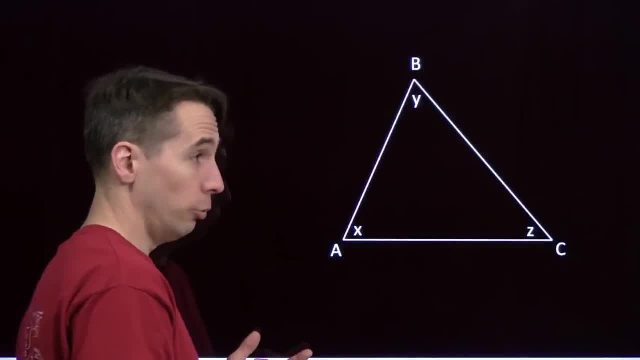 to—he wants me to look at the other problem, The other problem. Okay, Oh yeah, there's a parallel line here. Parallel line. These two lines are parallel, Harvey. Now, I don't see any here. You do. He sees parallel lines here. Do you see parallel lines here? I don't see parallel—through. 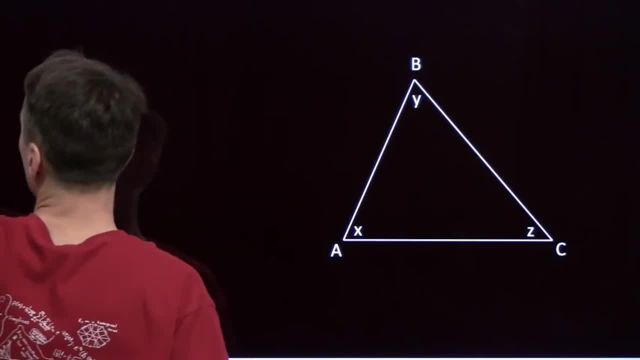 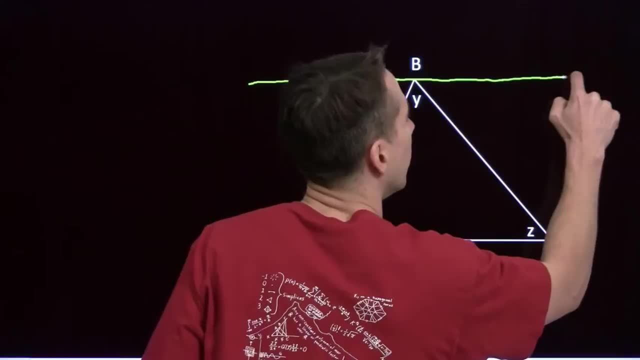 B parallel to AC. I'm going to draw it because I don't see it. Okay, Harvey, fine, I'll draw it in. There's your line, Through B, parallel to AC. Harvey, that's brilliant, My man's. 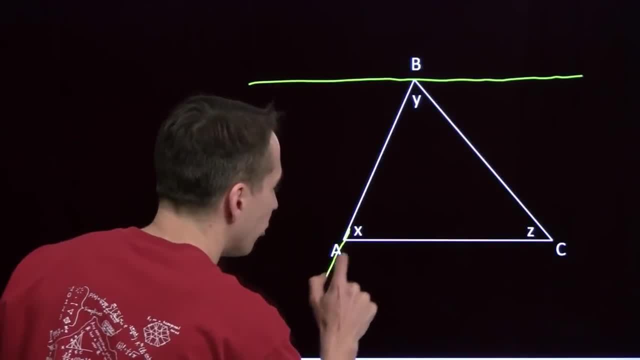 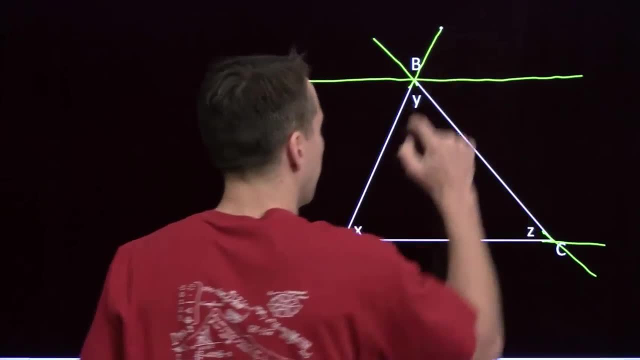 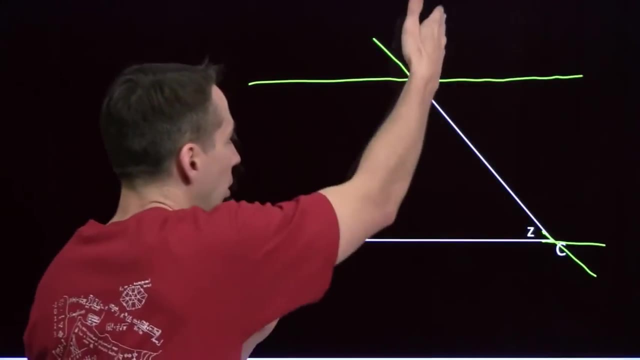 wicked smart, Just wicked smart. Check this out. Let's extend these lines a little bit. Extend these out And remember we have a set of four congruent angles. because these two lines are parallel and AB is the transversal. These four angles are congruent, So this up.